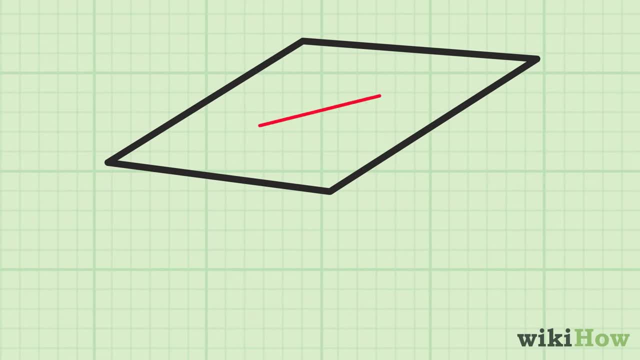 diamond-shaped rhombus. One is to measure the rhombus diagonally, from corner to corner each way. For instance, let's say your rhombus measures 10 centimeters across lengthwise and 6 centimeters across widthwise. Once you find the length of each diagonal, 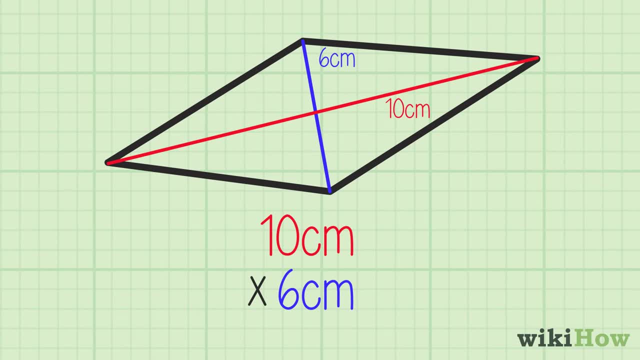 multiply the lengths together. In this case, 10 centimeters times 6 centimeters equals 60 centimeters. Finally, divide the result by 2.. Don't forget to square your units when you write the result, Since you're measuring the area. 60 divided by 2 equals 30.. So our rhombus has an area of. 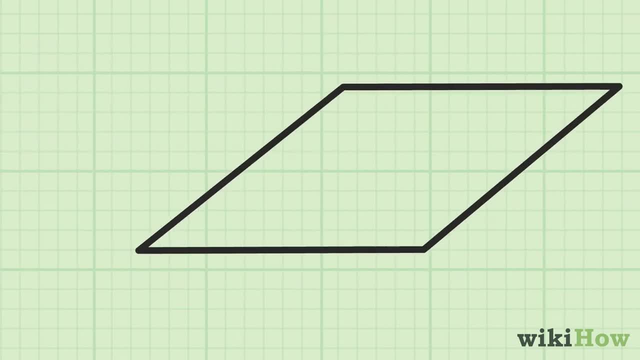 30 centimeters squared. Another simple method is to multiply the base length of the rhombus by its height. Measure the width of the bottom line of the rhombus, Then take a perpendicular measurement from the base to the opposite line at the top. Multiply the measurements together. 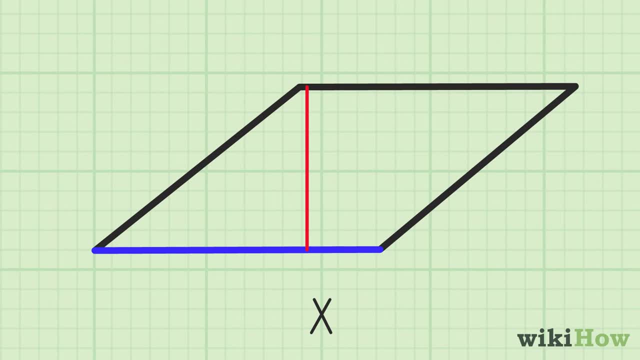 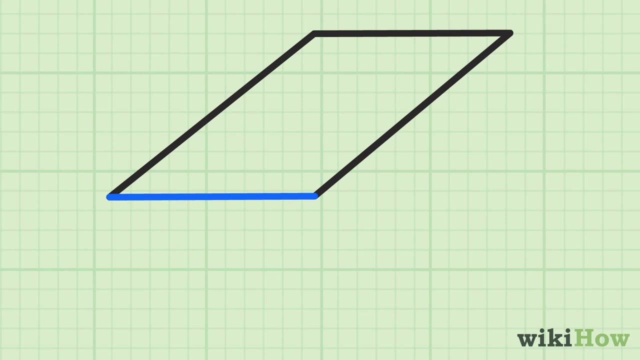 to find the area. For instance, if a rhombus is 12 centimeters long at the base and has a height of 8 centimeters, the area of the rhombus would be 96 centimeters squared If you only know the length of one side of the rhombus and one side of the angles. 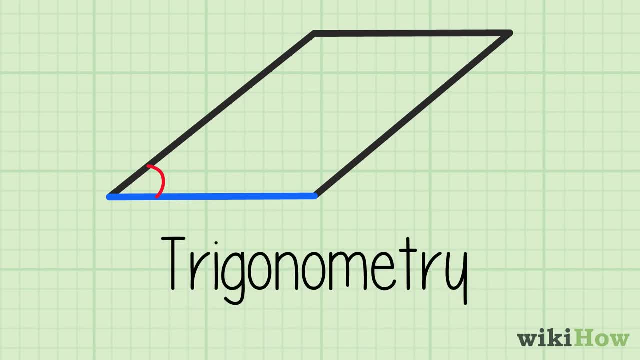 you can still figure out the area using trigonometry. To do this, square the length of the known side, then multiply the result by the sine of one of the angles. For instance, if the rhombus has one side with a length of 6 centimeters, 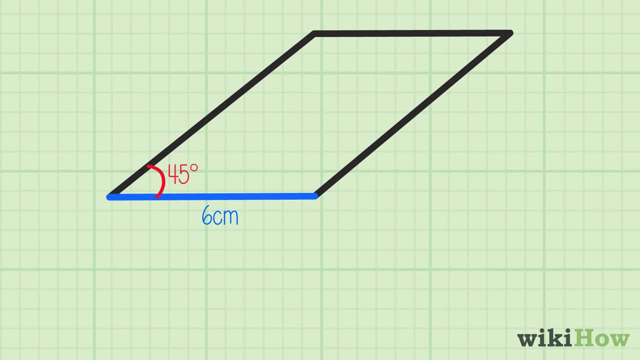 and you know it contains a 45 degree angle. the area would be 36 centimeters squared. x sine 45 degrees, or approximately 30.63 centimeters squared.